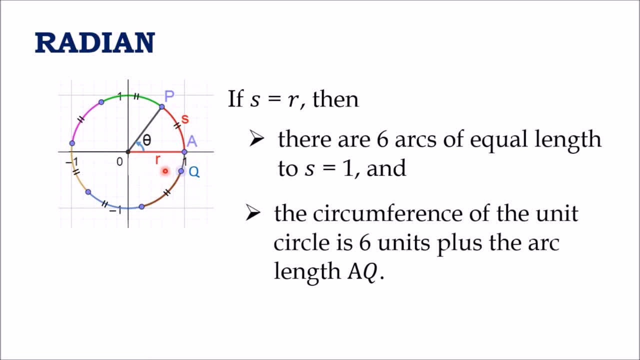 If S is equal to 1,, then R is equal to 1.. If S is equal to R, equal to 1 unit, then a unit circle has 6 equal arcs of length equal to S, plus the length of the arc QA or AQ. 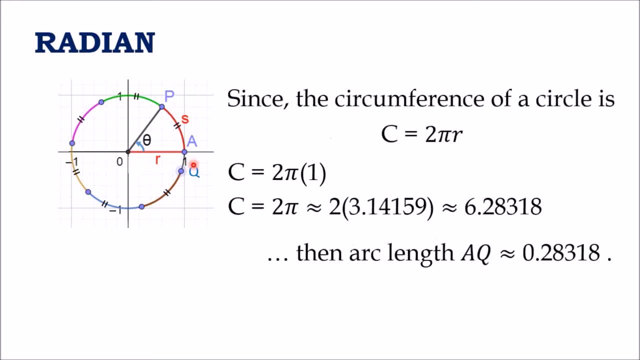 What is the length of the arc AQ? Since the circumference of the circle is computed through the formula C is equal to 2 pi R, then the circumference of the circle is computed through the formula C is equal to 2 pi R and the length of the unit circle is 2 pi. 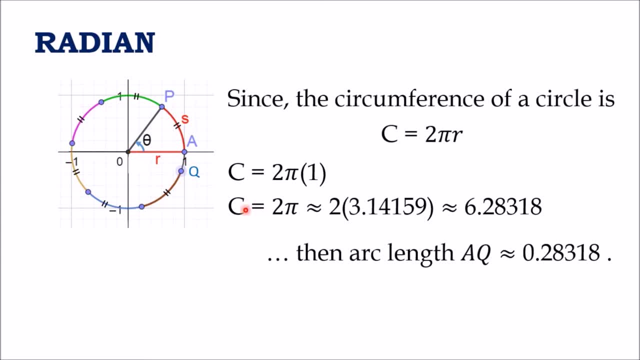 With this we can find the measure of the arc AQ. Since 2 pi is approximately equal to the product of 2 and the approximated value of pi, which is 3.14159,, then 2 pi is approximately equal to 6.28318.. 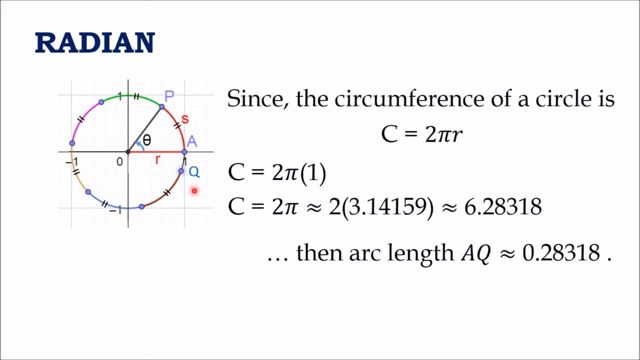 This clearly shows that the arc AQ is approximately equal to 0.28318.. What I am trying to emphasize here is that the circumference of the unit circle is equal to 2 pi. Solved through the formula C equals 2 pi r and through the idea of theta equals 1 radian. 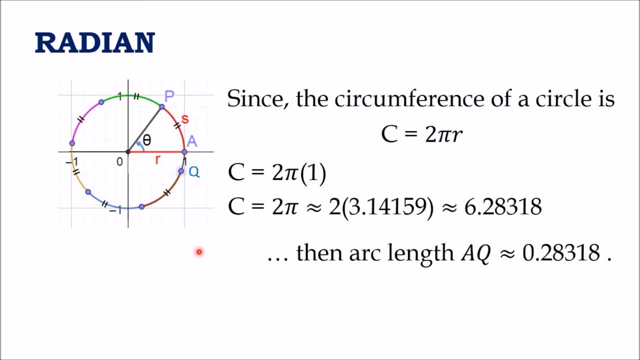 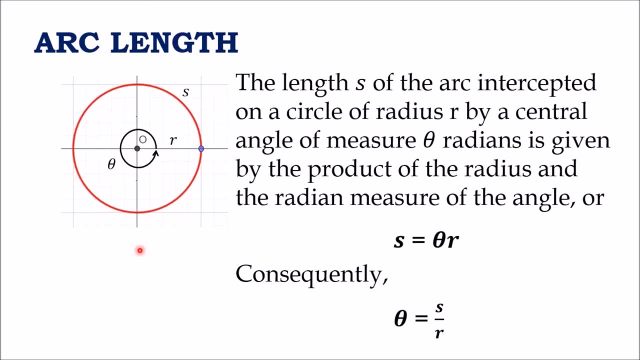 We will use these facts to know what is theta in radian measure when theta is fully rotated in a unit circle. Generally, when we find the length of an arc intercepted by a central angle theta, it is through the product of the measure of the central angle, theta in radian measure and the measure of the radius r. 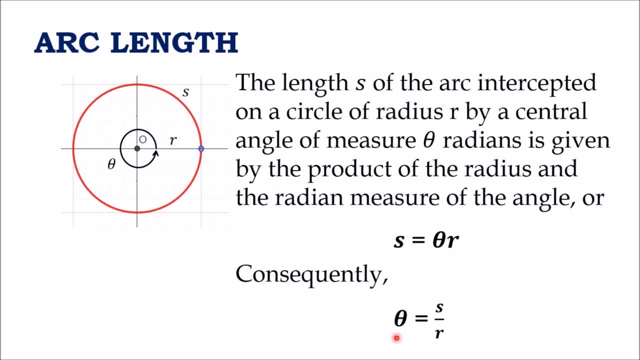 Now let's see how to find the length of the arc intercepted by a central angle theta. Consequently, the central angle theta in radian measure is the quotient when the arc length S is divided by the radius r. The arc length S is the linear measure.